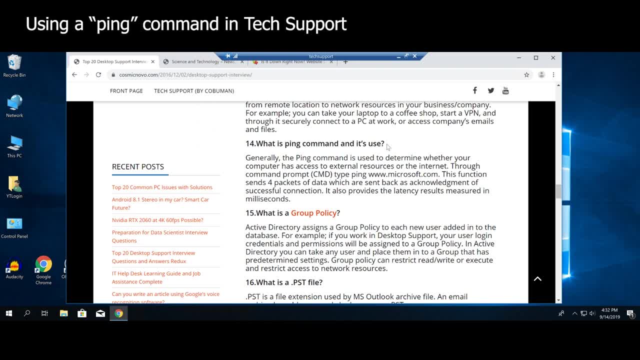 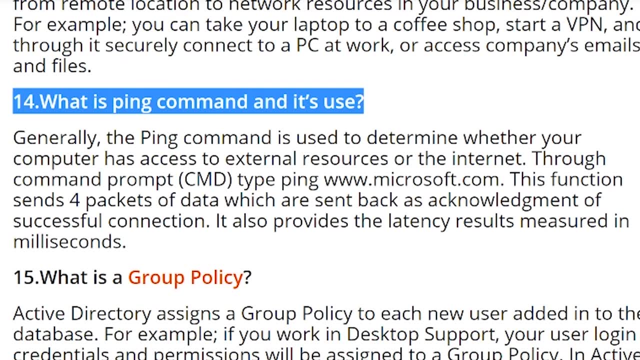 So it's easier to understand. So if you're doing tech support or desktop support or what have you, chances are you will be using PinCommand. So what is PinCommand and its use? I'm going to talk about the first part of it and explain the whole thing. 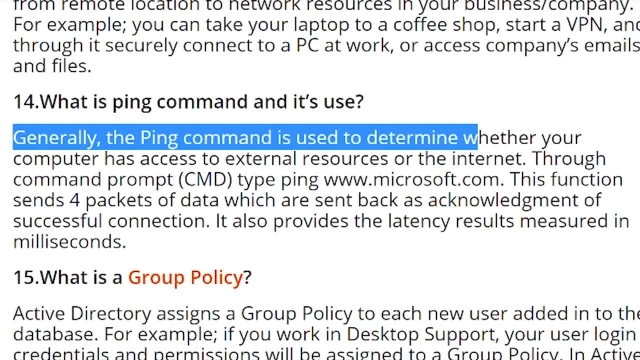 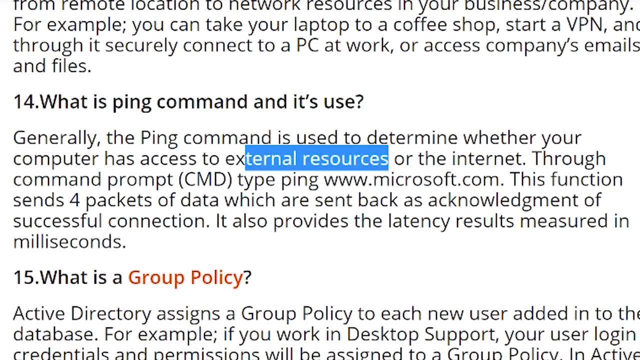 But my written answer here is: generally: the PinCommand is used to determine whether your computer has access to external resources or the internet. So anything that is considered external resources is anything that's outside of the connection of your computer. So let's say you're using a desktop PC at work or a laptop. 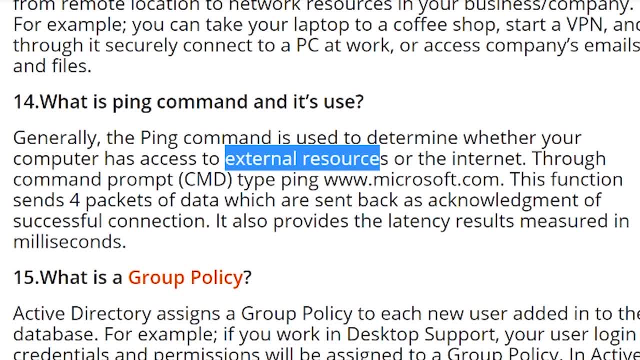 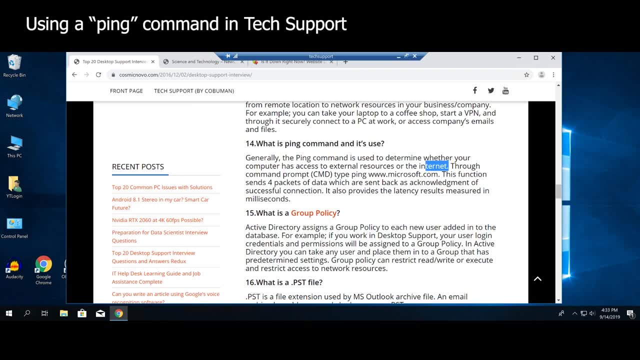 and then you're trying to access an external resource like a shared drive or a server or a website, whether it's internal or external, and you can't connect to it or there's an issue with latency or a lag of some sort. it's running slow. that's how PinCommand would be used. 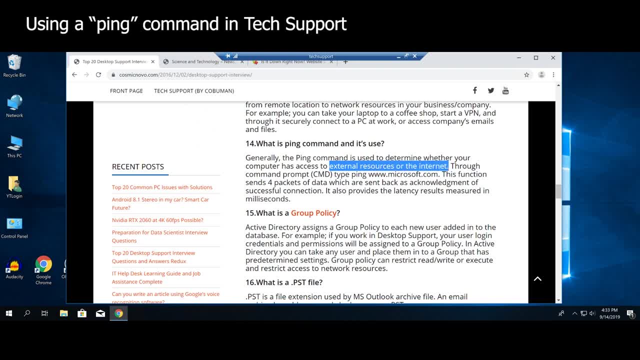 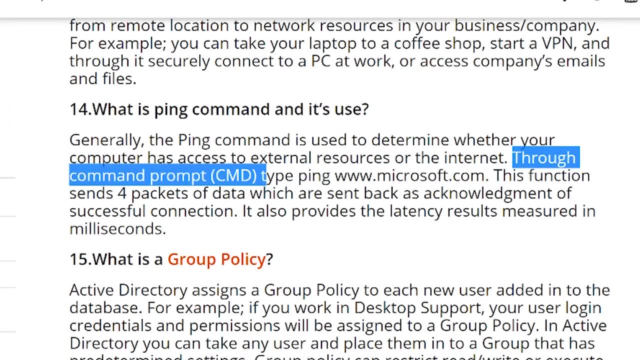 And all these things are considered as external resources, So something that your computer connects to over the network. Now, through command prompt, CMD, you can type in, for example, ping, wwwmicrosoftcom. And this is an example of a PinCommand. 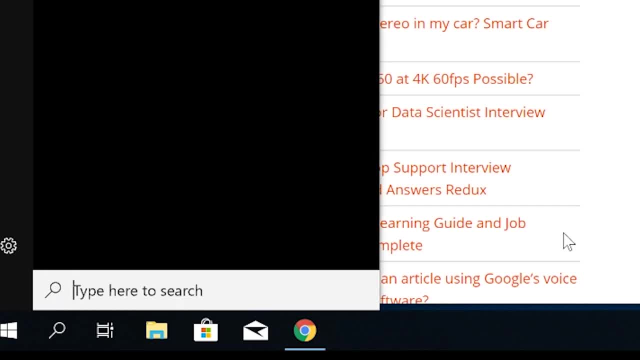 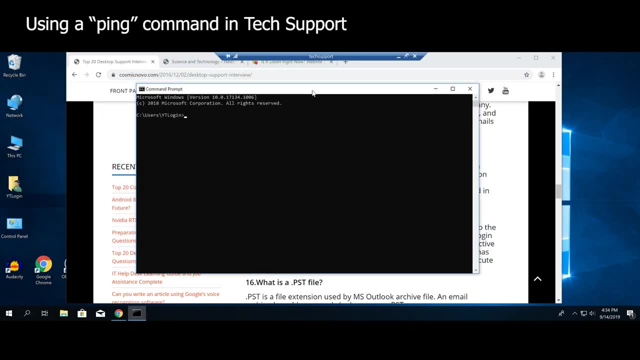 So let's go ahead and open up CMD. I'm going to open up command line, command prompt, or whatever you call it. I keep saying command prompt, command line. I use Linux too, so sometimes I forget which one is which. 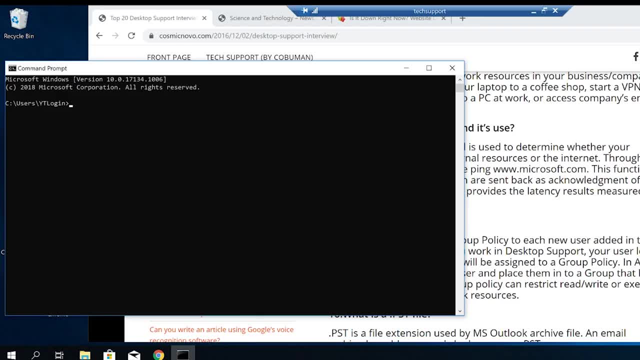 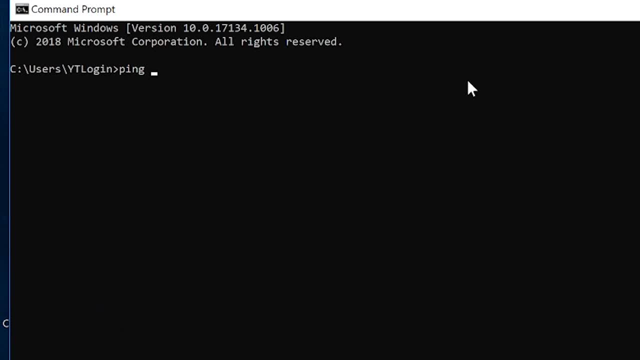 Anyways, we're going to use this example that we have here, and it's ping wwwmicrosoftcom. So let's see what happens when a normal working website is up and running and see the result from it. Did I misspell that? Of course I did. 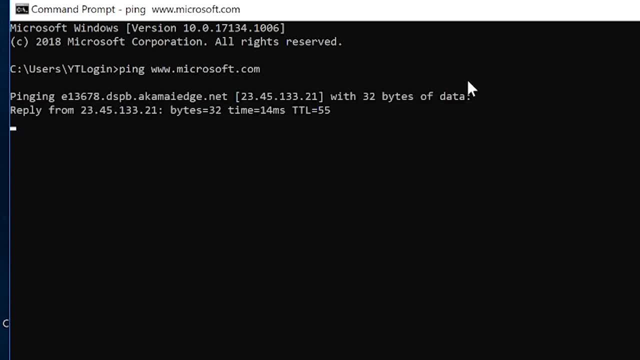 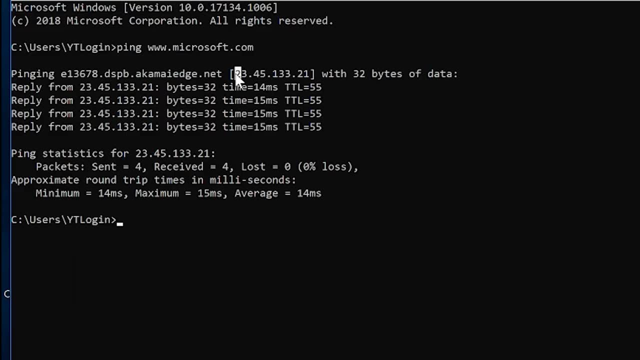 Microsoftcom. I'm trying to multitask here, so you will forgive me. Okay, so one of the first things that comes up that you will notice here is a number, which is an IP address, which is controlled by the DNS And the DNS. basically, what it does is 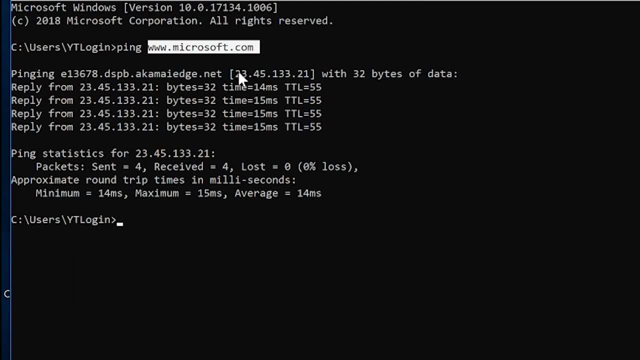 it takes a domain name, in this case Microsoftcom, and translates it into an IP address, which is the location of this website on a server. So the server for Microsoftcom is located at 23.45.133.21.. So that's the IP address for the server of the server for Microsoftcom. 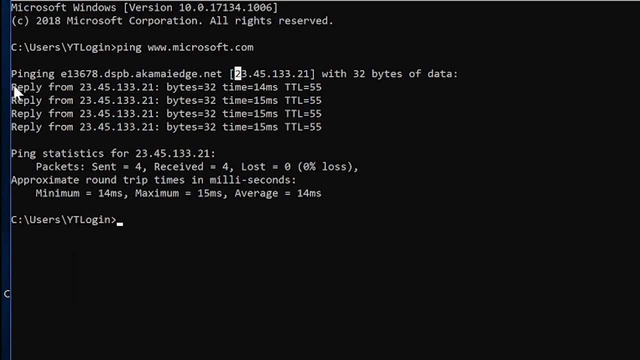 Okay, so now these are real results of the ping command for a normal running website. that is up and running and there are no problems. So what happens is ping command sends four packets of data, So you can see here that it sent four packets. 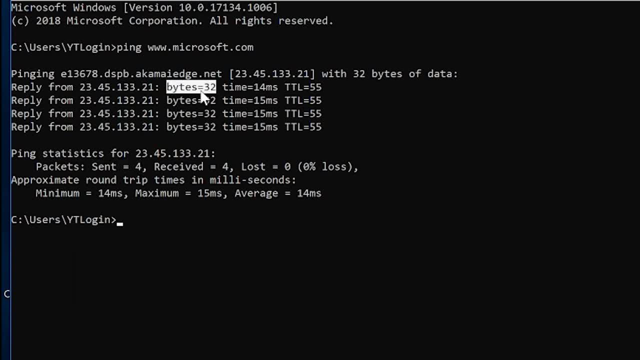 They are a size of 32 bytes And then it waits for a response and how long it takes to respond, which is shown here in milliseconds. So this is the first attempt from of the ping this IP address And we can see that the response time here. 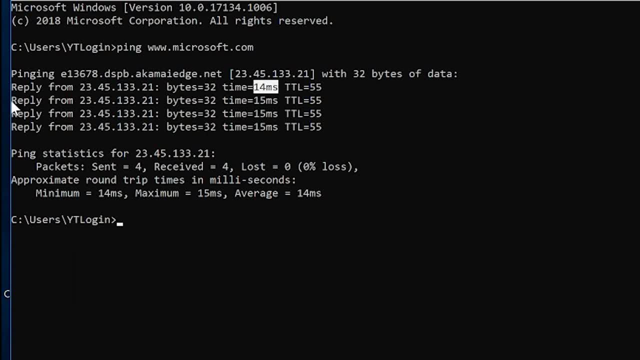 that it took 14 milliseconds to respond. And then the ping command does it again, which is the second time, And this time it replied in 15 milliseconds, And then the third time, also 15 milliseconds, And then fourth time, also 15 milliseconds. 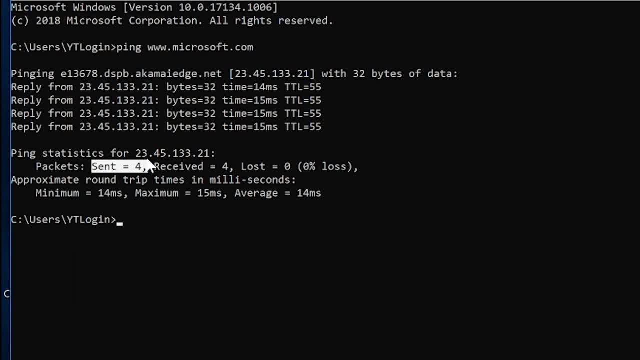 Hence four packets sent right. Very, very easy to understand. But of course, for it to actually respond, for it actually to have a response of any sort, it has to send back four packets as well. So you can see here that the server at 234513321,. 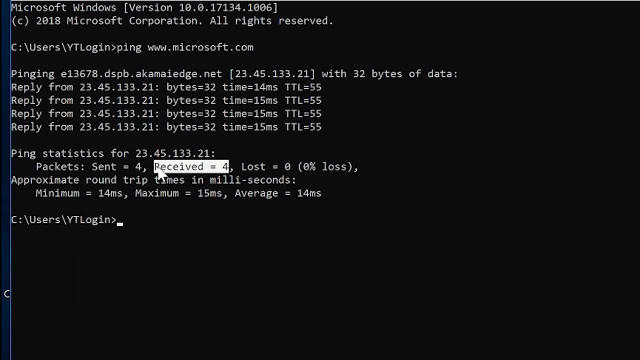 also sent back four packets which were received at the same size, And then we can see that lost zero. that means it was successful, That means none of the packets failed, that all the four pings were successful. That's an example of successful. 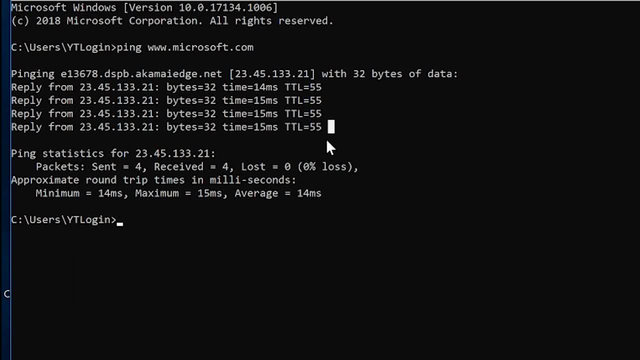 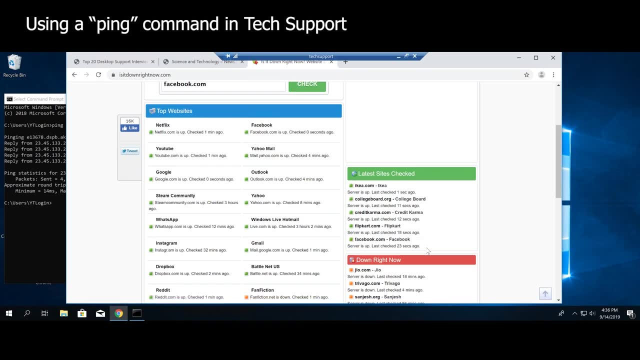 Again, here we're going to go to the ping command. We know everything is okay with this website, So let's go find a website that doesn't work. So I went to this website and this website tells you of some of the big websites that are down. 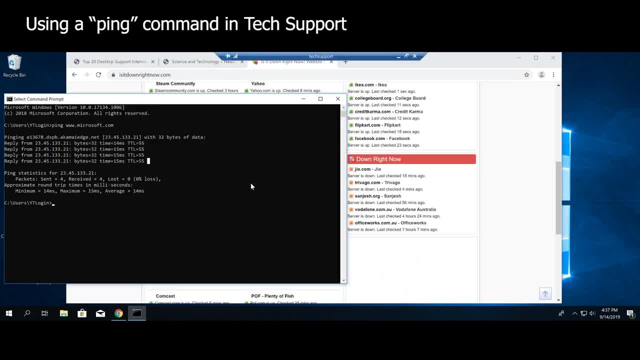 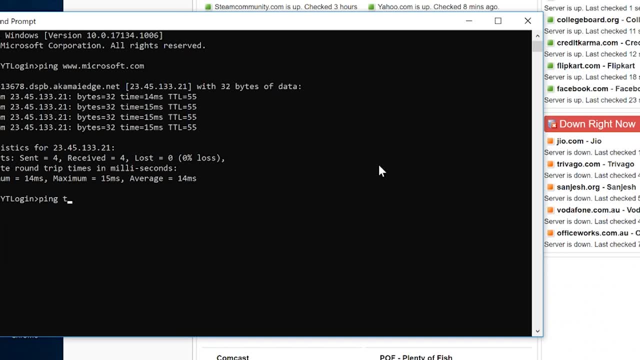 So let's pick a random one here. Let's pick trivagocom here. That's a safe website. We're going to type in, ping trivago. Well, let's do www dot wwwtrivagocom dot-com. now, if this website is down, like it says it is, we're going to get some. 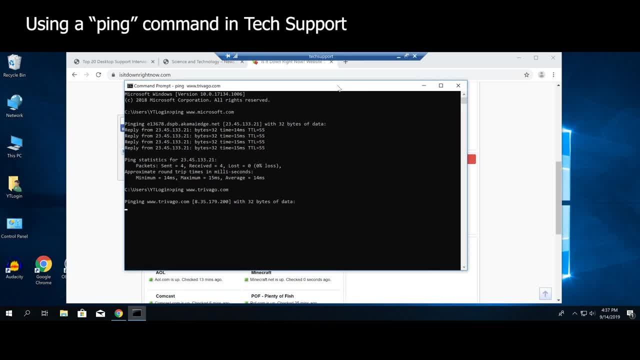 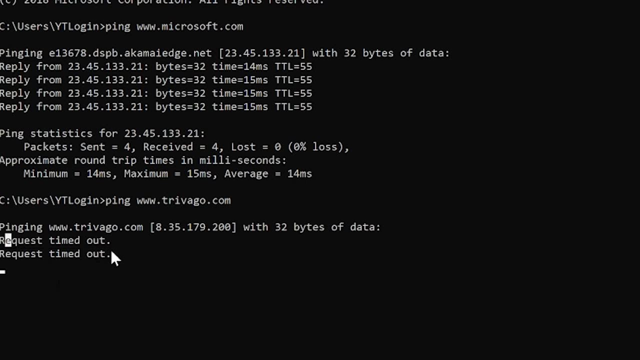 negative results, which would be eggs. good example of use of how you use a ping command and how to help you troubleshoot the issues. so so far, we can see that it's timing out. what does that mean? that the first packet was sent and it didn't connect. it waited a certain amount of time, didn't connect to the. 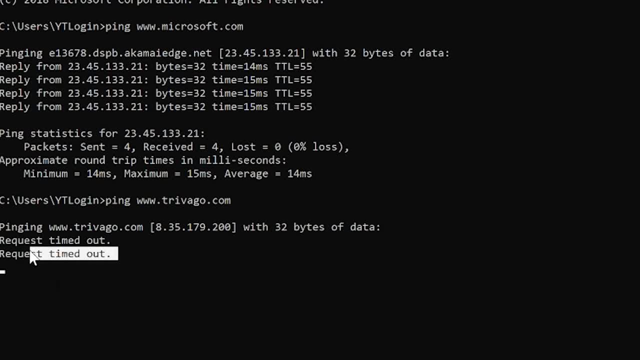 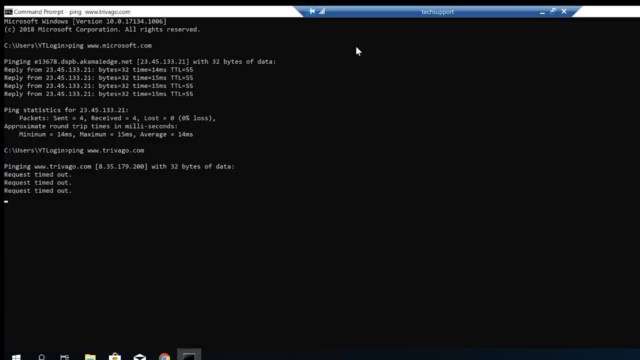 server, or the server didn't reply, I should say, and they timed out. and then the second time as well. I'm sorry. first time, second time and we're waiting for the third one. third one timed out. I'm sorry, I didn't mean to go all full. 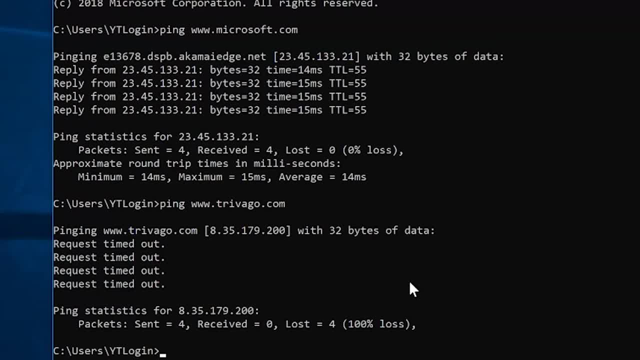 screen here. let me kind of move some of this stuff out of the way so it's easier to see and we can see that all four packets sent timed out. that means that server, just we, you know the, the ping, you know waited, waited. you know we waited. 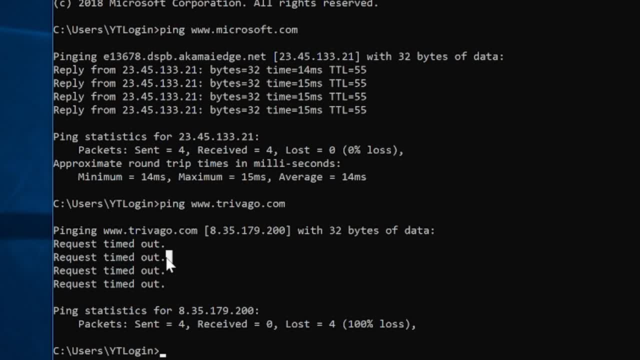 and the server didn't reply. respond timeout: there's only a certain amount of time ping command will wait for a response, and that's what happened, and we can again see here that four packets are sent so and then zero received, and in this example, trivagocom. 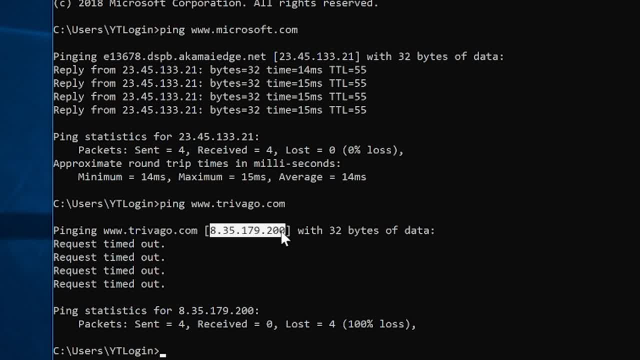 is located at this IP address. that's the server, that's the web server for the trivagocom, and now we can see that we sent four, we waited, we waited, nothing happened. we received zero because it's down, and then we lost four. that means we sent four and they never came back, which gives us one hundred percent loss. 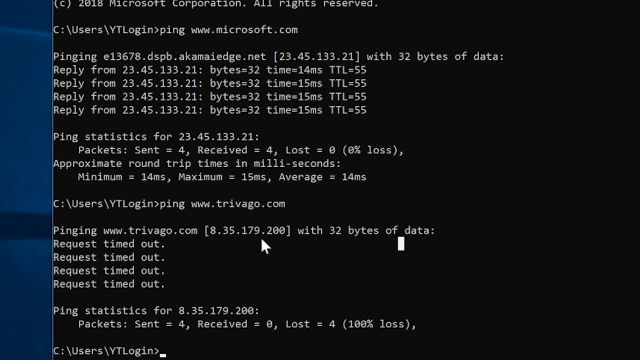 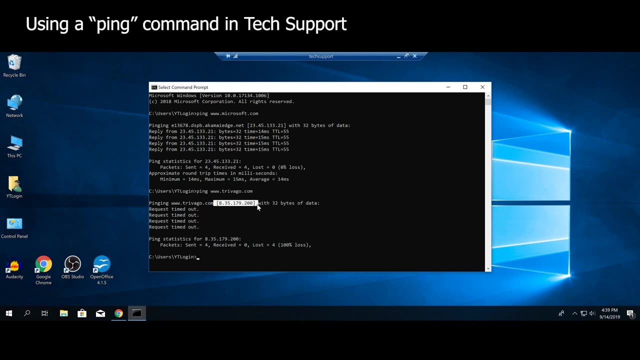 off packets. so how does this help us? well, for, for one thing, we know the website is down, or you know a server that you're trying to access at your job is down. right, we can. you know web server or some, some other network component, some other network resources, you know, if you have the 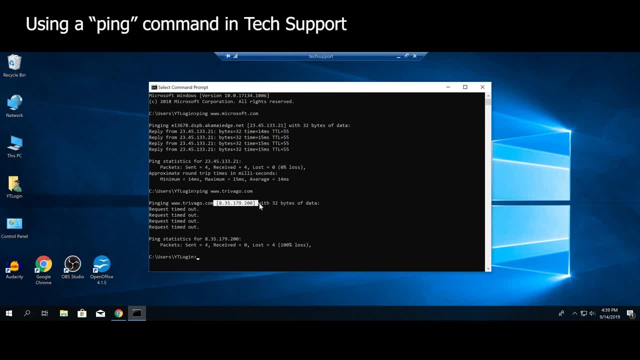 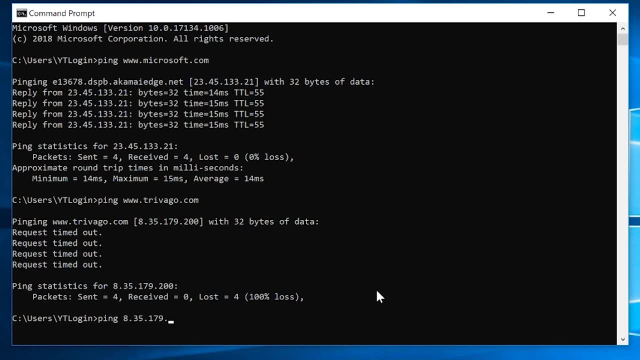 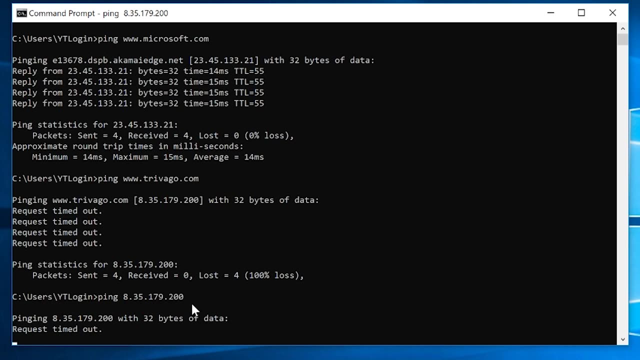 name for it or the ip address. you can just ping the ip address if you wanted to. you can just type in: ping you know, ip address 35179.002.200. and here we go again. we're pinging trivago's server again, except we're just directly bypassing the domain name. now we're bypassing the dn. well, we're not. 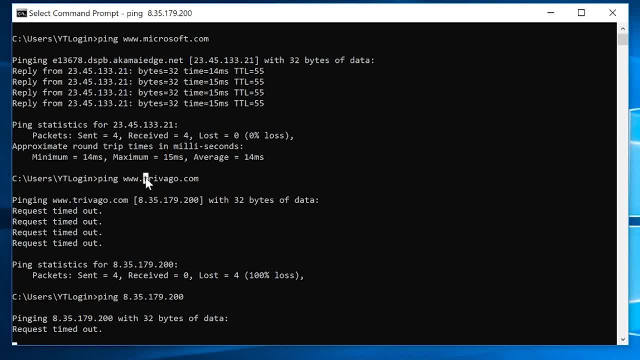 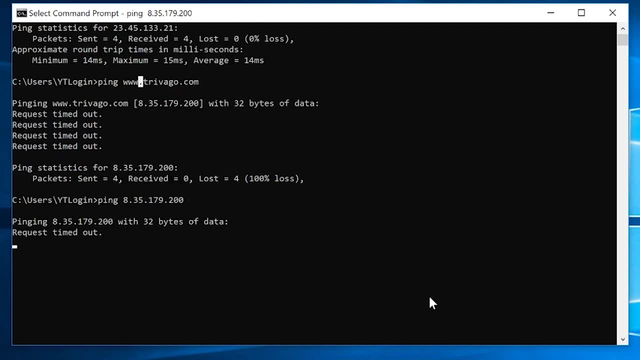 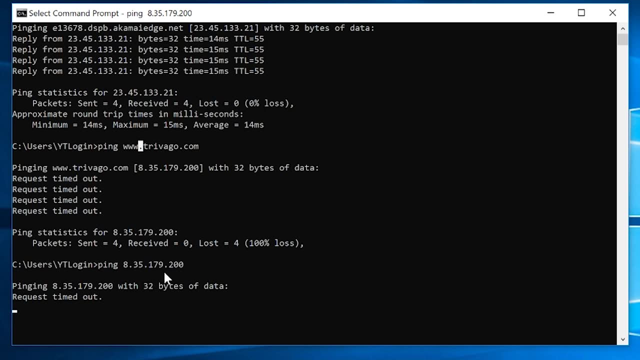 necessarily bypassing, but we're bypassing the uh domain name, we're going directly to pinging the server itself and again it's timing out, which is another indicator that the website is down. so, going back to the uh, my question of how does this help us, aside from knowing that the website is 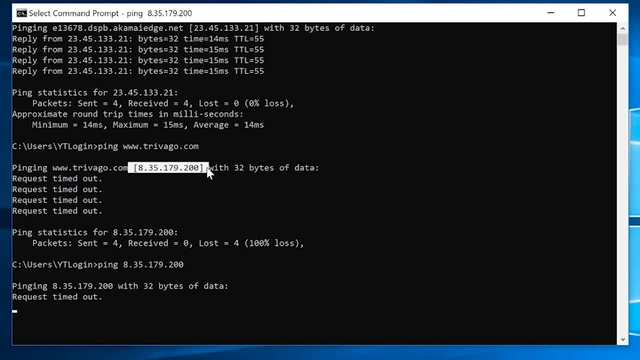 down. so if it's an external website, what we would have to do is find the web, uh webmaster for it or a person who has access to the server. same thing goes for if it's an internal website. so let's say your business or the business that you work for has some kind of internal website. 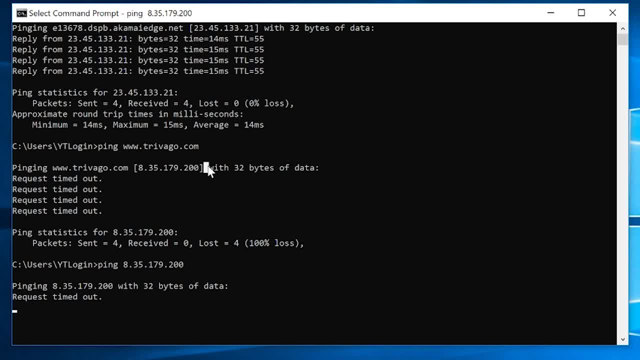 that everybody goes to, everybody uses it. you know this and that and you know you don't have necessarily access to it. you would find that webmaster and contact them. so how would you go about that? well, if you know who the owner of trivagocom is, you would contact them directly, obviously. but if you don't know who the owner is, 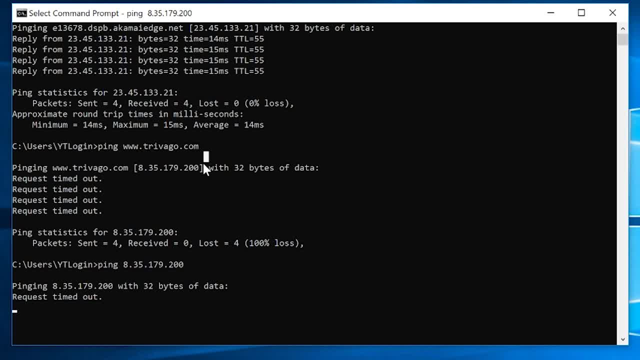 based off that, the name of the trivagocom, based off the domain name, you can see who the owner is of this ip address, and this is something that this is something that your company would provide this to you if you're doing tech support, so you would basically have a tool that lets you tool, or 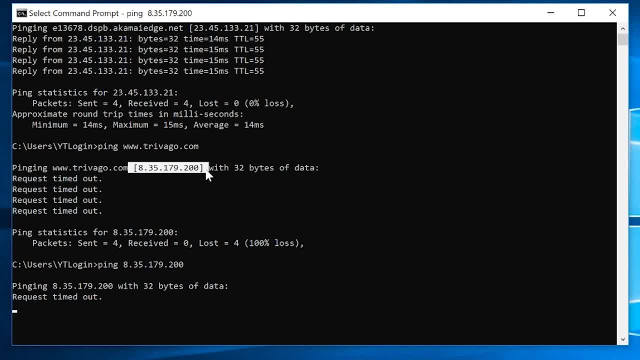 you know some kind of notes or something i don't know. this is all depends on. this varies from place to place, you know, but for example, at my main job, i know i will know who owns this ip address. so not only can i look up to see who owns trivagocom, 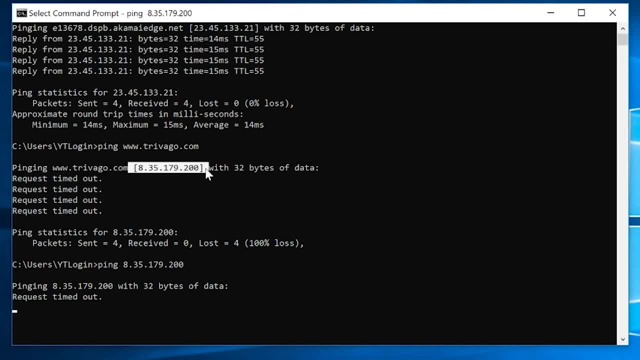 for example, i can also look up who owns this ip address and then i would contact that guy who is the owner of this ip address, or a guy or a gal or whatever. um, i would contact them, say, hey, this website is down. but the only time i would contact them is if they're not the owner of this. 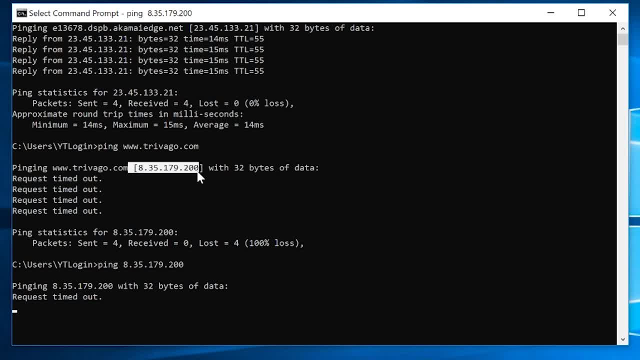 ip address. so the only time i would do that is if i don't have direct access to this. so let's say: if this is a server that i have, you know that i'm running and everybody in the business here is using it as just a storage location, you know, let's say: this is just a web server that hosts. 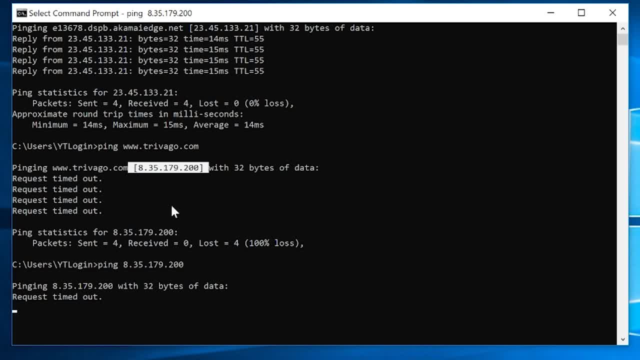 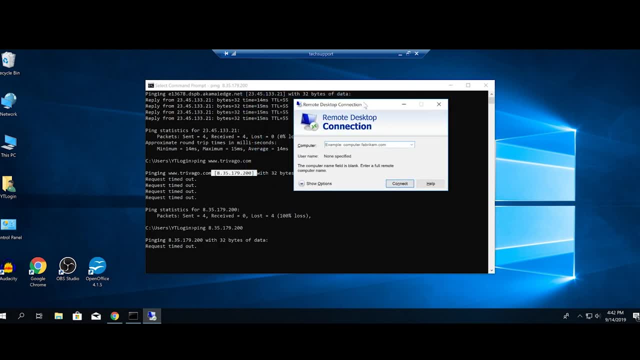 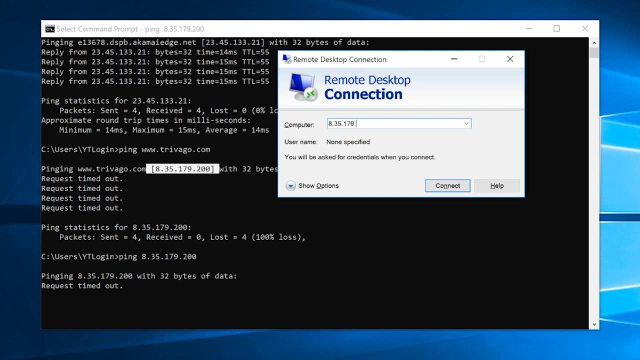 files for everybody in my building that i support. well, i would simply just try this. you know, if i don't have physical access to it, i would open up remotely and i would just try this, and i would desktop connection type in 8.35.179.200- see if i can connect to it. you know, and it's going to fail. 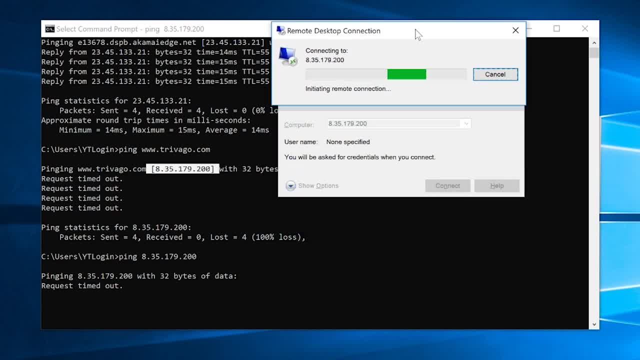 because obviously i don't have access to it, and you know that's okay. but if i have physical access to it and i know where it's located- in the data center or in a server room or whatever it is- chances are this: you know, this server might be just turned off. 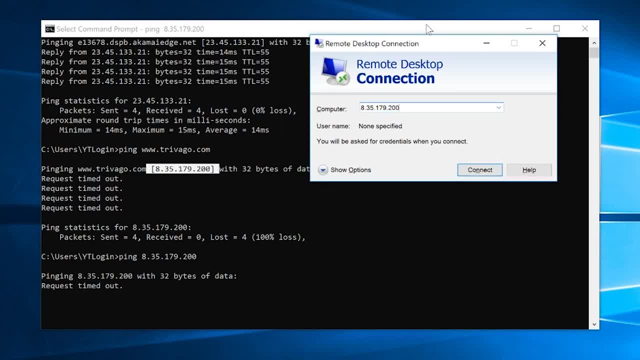 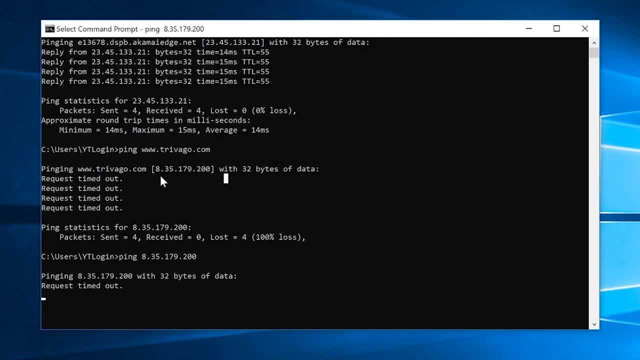 or you know, there might be something else bad with it. but at least i will know that there is something wrong going on by using the ping command and that will get me to either me fixing it or finding who can fix it. and that's how you would use ping command in a business environment. 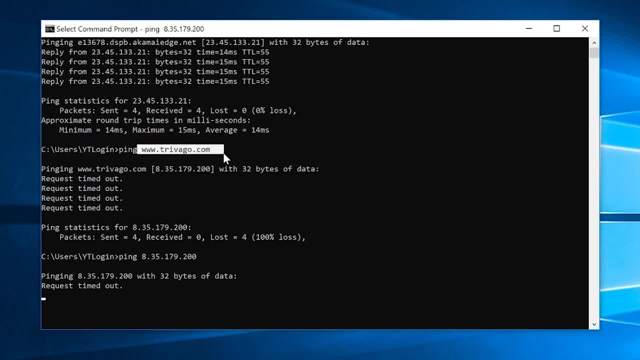 you know, if you're doing more network network administration support, you can use traceroute and find out more about this, but i will save that for another video, so be sure to subscribe. all right, guys, i hope you like this easy to follow video. please share this video with your friends. i really appreciate. 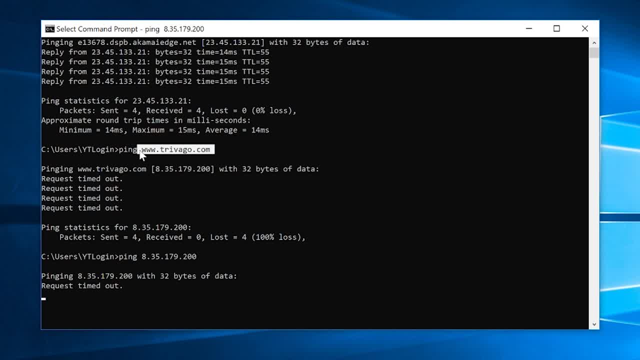 it. it really helps me, uh, helps help support my channel, basically. so thank you so much. please leave a like and i'll see you next time. bye. 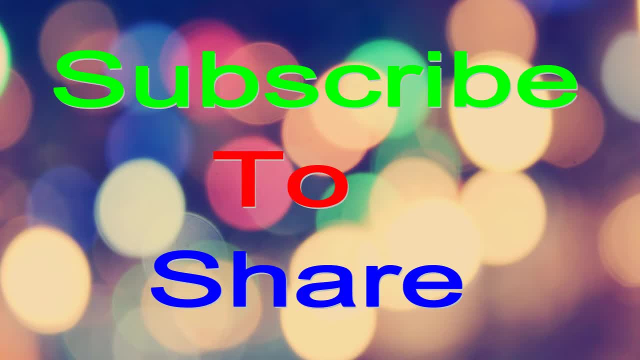 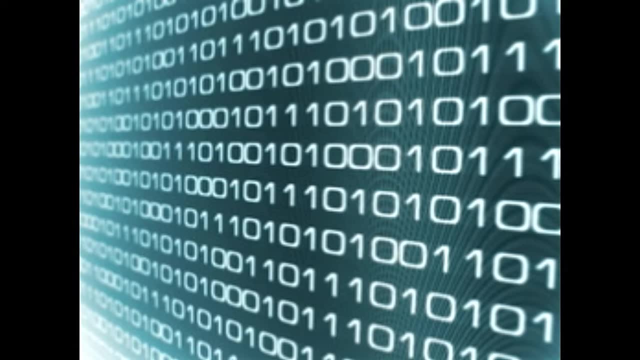 Thank you for watching the benefits that it provides every day For those who deal in the business of protecting information using information technology. cryptography is akin to the holy grail. Initially, it was only used by the military to decode enemy messages, but today is being used in things more mundane such as email. Cryptography deals with all. 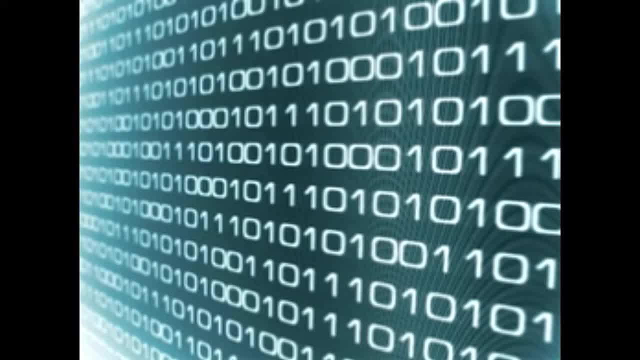 aspects of secure messaging, authentication, digital signatures, electronic money and other applications. It protects a message or file from being read by an eavesdropper who has no other means of access to either the original text of what is protected or the key with which it is encrypted. When a 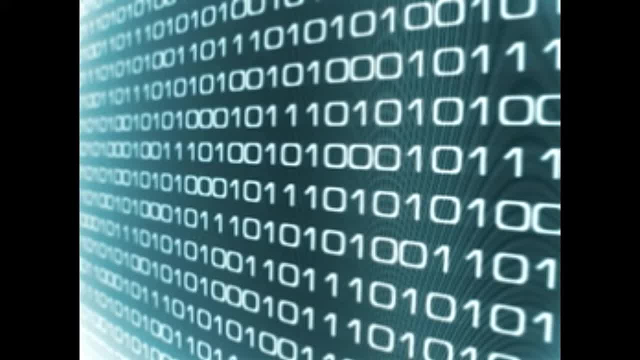 message is sent to someone, it is converted into undecipherable code so that no one other than the intended reader would know what is written. Once the message reaches the intended recipient, he will require the program that decrypts it. Julius Caesar was a master of a primitive.